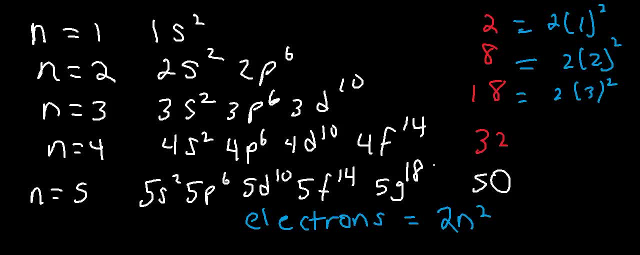 which is 2.. When N is 1, it's 2 times 1 squared, which is 2.. When N is 2, it's 2 times 2 squared, you get 8.. When n is 3, 3 squared is 9 times 2,, that's 18.. For 4, 4 squared is 16, you. 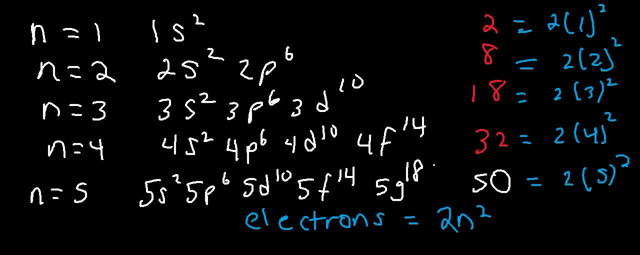 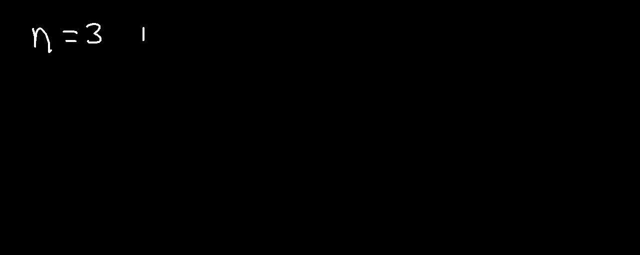 double it, you get 32.. 5 squared is 25 times 2, you get 50.. So that's how you can find the maximum number of electrons in any energy level. Now let's consider the second case. Let's say, if you're given the value of n and the value of ms, Whenever you're given the 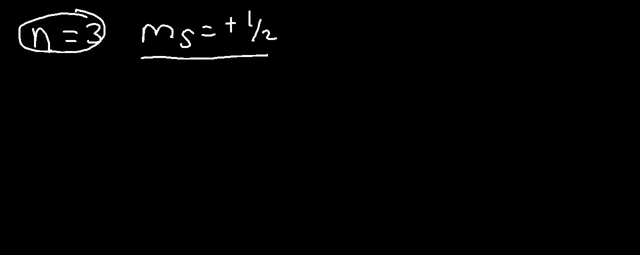 value of ms. it's simply half of the previous quantum numbers. In the third energy level we know that there is a maximum number of 2n squared electrons, which is 18 electrons. Half of the 18 will have an electron spin of plus 1 half, and then the other 9 will. 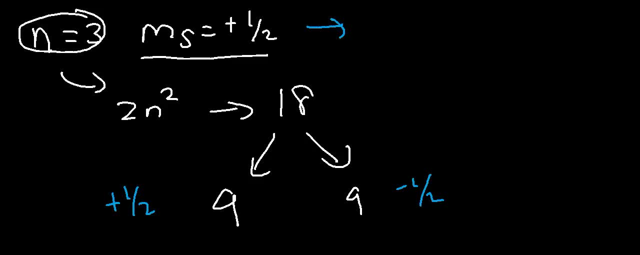 have a spin of minus 1 half. So the answer is half of 18, it's 9 electrons that will have these two quantum numbers. That's the second case. So just for another example, let's say if n is 10 and ms is negative, 1 half, We know. 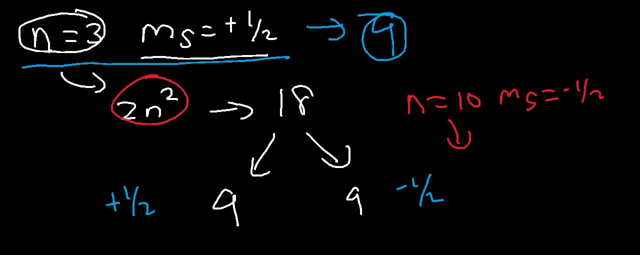 based on the equation 2n squared, that you have a maximum of 200 electrons in the tenth energy level. However, half of those will have a spin of negative 1 half. so the answer will be 100.. The third case is when they give you the value of n and the value of m, The 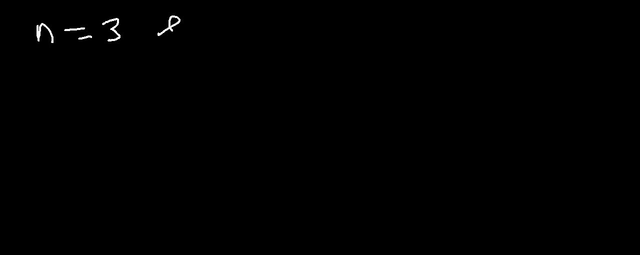 donuts upon the instant. ediyorum is 2.. When the interest rate and L is 2, we get aむn ore, which is zero For the pm sublevel. l, that's one. For d, We get 18, we get 1.. For F, We take L. This means the maximum of. electrons. For s, we need to know that L is one, For p, a maximum of 1, so, given l is two and l is zero, For s, we need to know that L is 0.. For d, we need to note the l For f. a love. 1's for f, 0's for l is 1.. For d, l is 1.. For f, l is 2.. So what this means is that when n is 3 and L is 3, we have the 3d sub level, And in a 3d sub level you can have a maximum of. 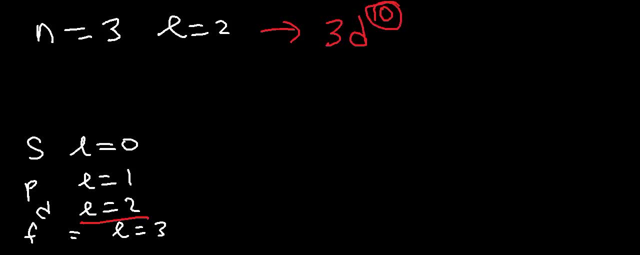 answer is 10.. For the sake of practice, let's say if n is 4 and l is 3.. This correlates to the 4f sublevel and the f sublevel can have a maximum of 14.. Let's say if n is 2,. 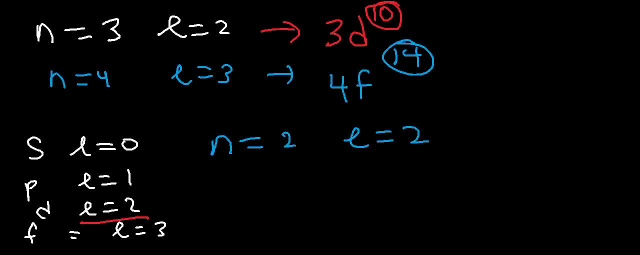 l is 2.. Now this is impossible. l has to be less than or equal to n-1.. So when n is 2, l can be 0 or 1. It can't be 2.. So if you have quantum numbers that aren't allowed. 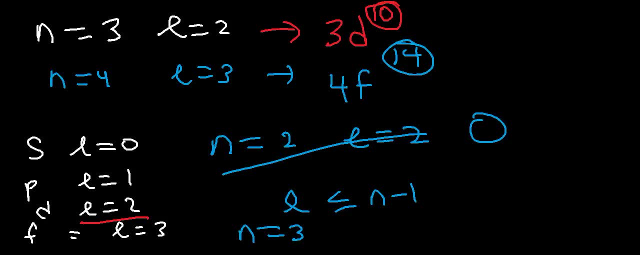 the answer is 0.. Let's say, if n is 3 and l is 1. This correlates to the 3p sublevel right And there is 6 electrons in the p level. So there are 6 electrons that can have these. 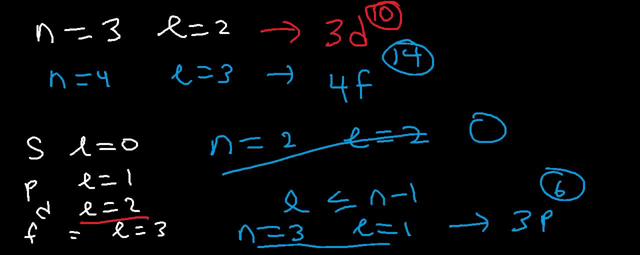 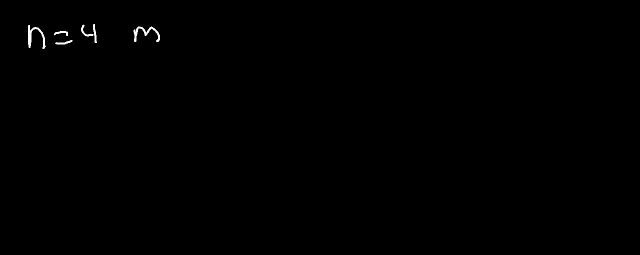 those two quantum numbers. Now let's look at the next case. let's say, if you're given the value of n and m-l- Subtitles by the Amaraorg community- What is the maximum number of electrons that can have those two quantum numbers? 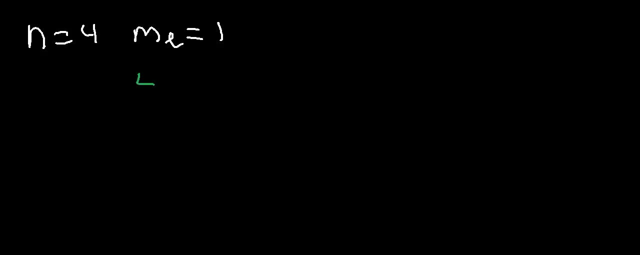 Well, let's make a list of all the sublevels in the 4th-inch level. We have 4s, 4p, 4d and 4f. There are four sublevels in the 4th-inch level. 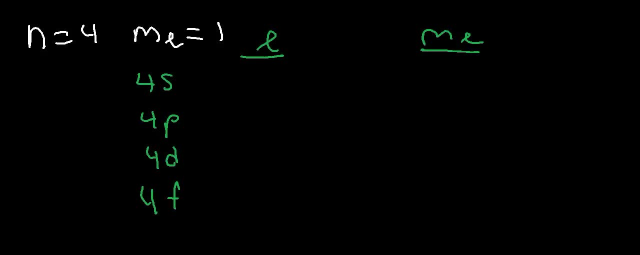 We're going to list the values of l and ml. For s, we know that l is 0.. It's 1 for p, 2 for d, 3 for f. When l is 0, ml has to be 0. 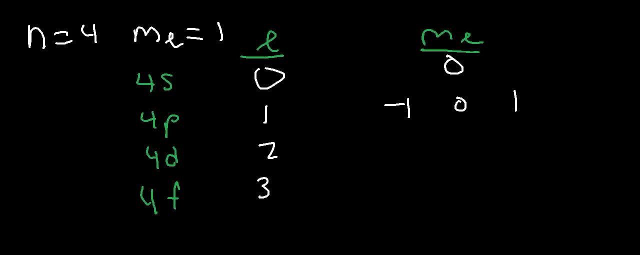 When l is 1,, ml can vary between negative 1 and 1.. Likewise, when l is 2,, it can vary between negative 2 and 2.. So ml can only be between the range of negative l and l. Now, each of these sublevels has an n value of 4.. 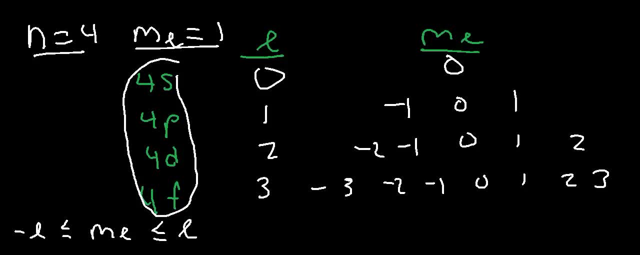 However, only some of them have an ml value of 1.. And that's these numbers. here The ml values corresponds. it identifies the orbital within the sublevel. The 4th sublevel has one orbital. The 4p sublevel has 3.. 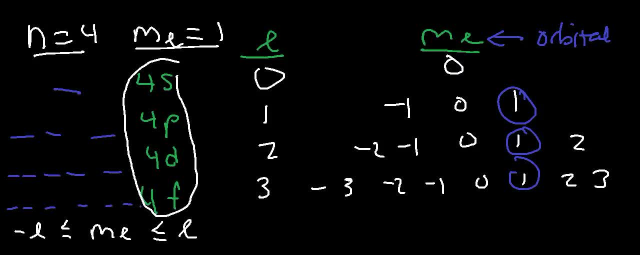 4d has 5. And f has 7. And each of these numbers corresponds to that In every orbital you can have a maximum of two electrons. So therefore there are six electrons that have these two numbers. So the answer is 6.. 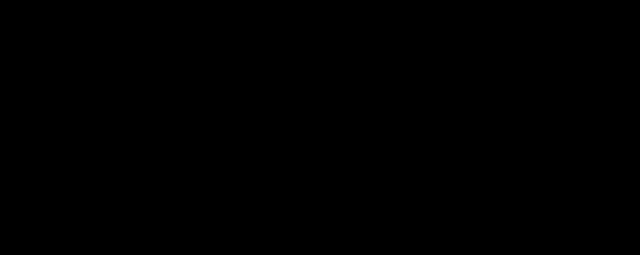 Let's try another example for the sake of practice. Let's say: if n is 5 and l is 3.. So for the 5th energy level, we have 5 sublevels: 5s, 5p, 5d, 5f and 5g. 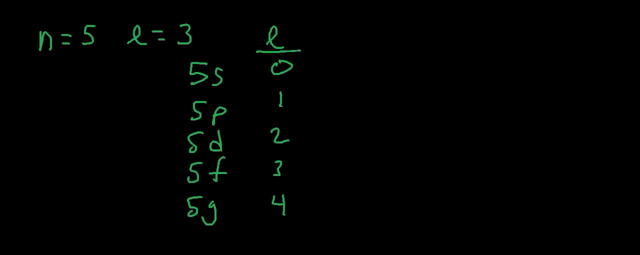 And these are the values of l that correspond to those sublevels levels and the values of ML. now we need to know which of these, all of these sub levels, are part of the fifth energy level. but not all of them have an L value of three, only these two. 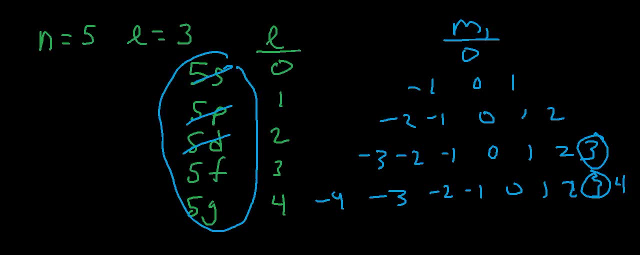 and every orbital can hold two electrons. so therefore there is a total of four electrons that have those two quantum numbers. actually, this is not supposed to be out. this is supposed to be ML, which has a value of three, and there are four electrons that have that. if n was five and L was three, then this would be the. 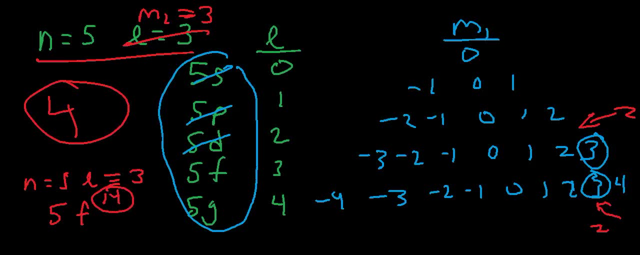 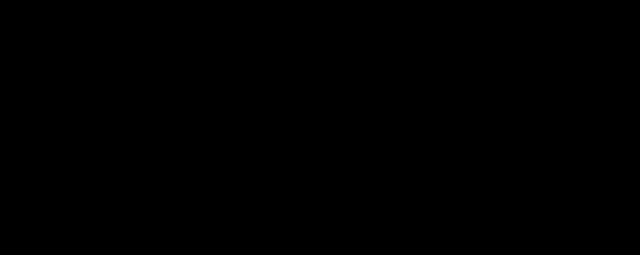 5f orbital, which can have 14 electrons. but I don't know if you can see it on the screen, but if you can see it on the screen, I meant to put ML in there. all right, the next case, let's say if we have, if n is three, L is two and ML is one. well, this part. 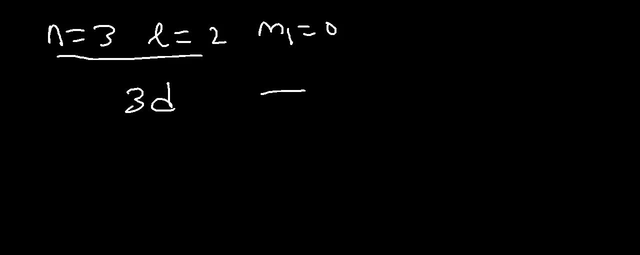 corresponds to the 3d sub level and D has five orbitals. because L is two, it can. these numbers can vary between negative two and two, and we're focused on the orbital that has a value of zero. there are two electrons in an orbital, so whenever you have these three quantum numbers, the answer is: 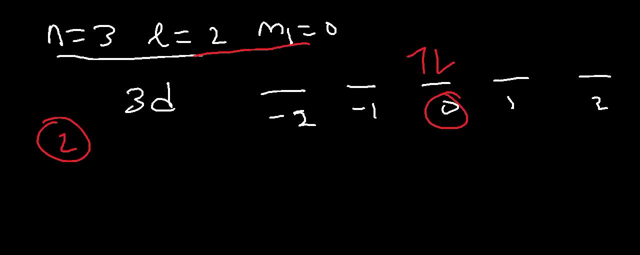 always going to be two, because we're specifying a specific orbital. now let's say: if it's not allowed. for example, let's say: if n is three, L is one and ML is two. do you see the arrow with this? these quantum numbers, ml can never exceed L. if L is 1, oriteitms von piu 2. 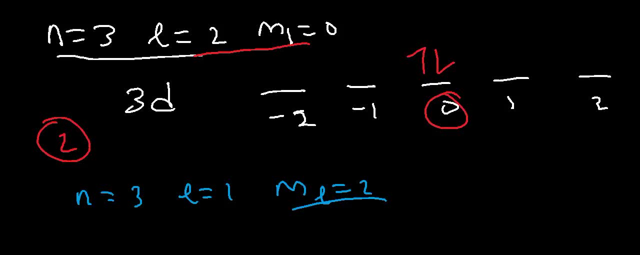 see the error with this. these quantum numbers, ml, can never exceed L. if ML can never exceed L, if the answer is n1, it can never exceed l. if n isワ, the answer is n2, ML can never exceed L. If L is 1, ML has to be between negative 1 and 1.. 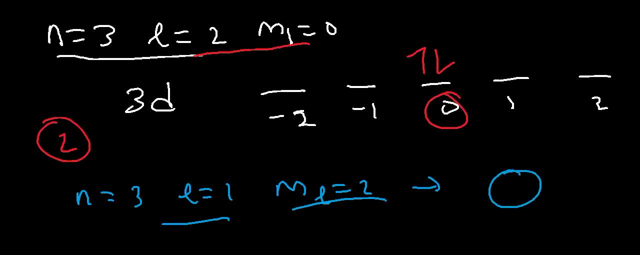 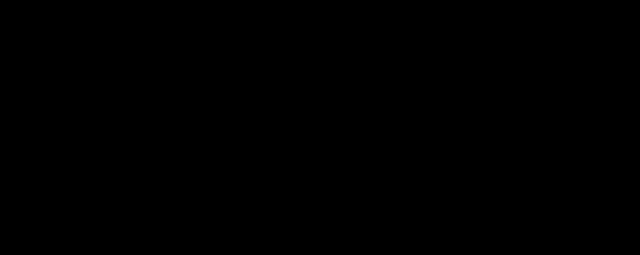 So when you have quantum numbers that are not allowed, the answer is 0.. If it's allowed, it's going to be 2.. So now let's go over the next case. Let's say: if N is 4, L is 3, ML is 1, MS is minus a half. 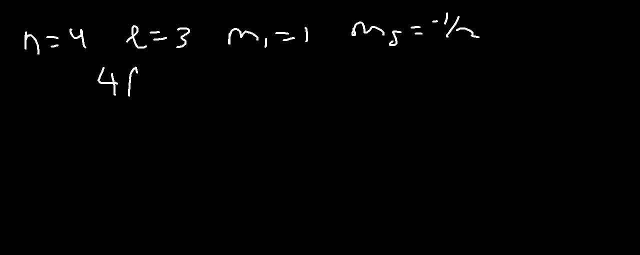 So we know that we have the 4F sublevel, which has 7 orbitals, And we're focused on the orbital that has a value of 1 for ML. Now, there are 2 electrons in this orbital, but only one of them has a spin of minus a half. 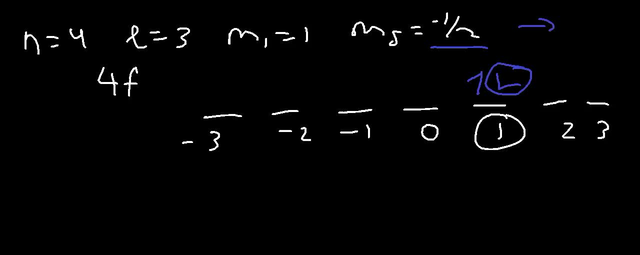 Therefore, when you have all 4 quantum numbers, the answer is always 1 electron. If those quantum numbers are less than 1, then you have a spin of minus a half. If it's not allowed, then it's 0.. 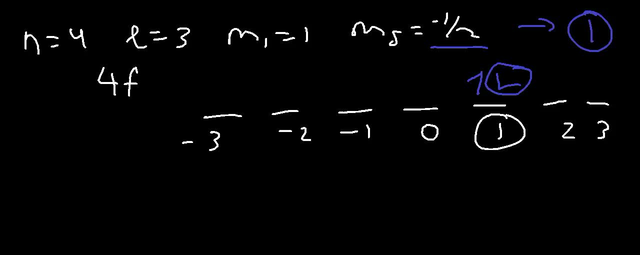 This is based on Pauli's Exclusion Principle, which states that no 2 electrons can have the same set of 4 quantum numbers. These quantum numbers, they identify a specific electron. They are part of an identification system. Let's try another example. 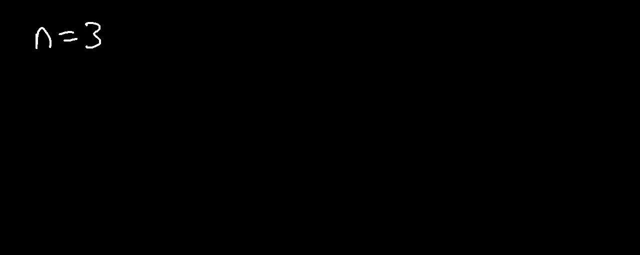 Let's say, if N is 3.. L is 2, and MS is negative, a half. Whenever you have the value of MS, look at the previous two. It's simply half of that. When N is 3 and L is 2, we know we have the 3D sublevel, which can have a maximum of 10.. 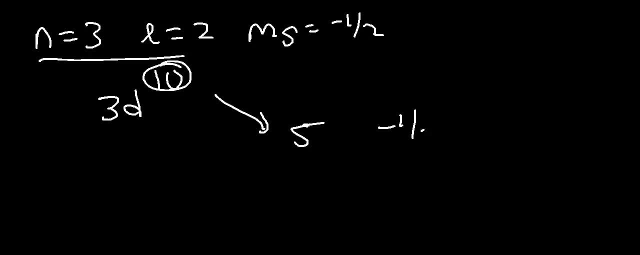 Therefore, half of those 10 electrons will have a spin of minus a half. The other 5 electrons will have a spin of plus 1 half. So the answer is 5. It's half of what this number is. Now let's consider our final case. 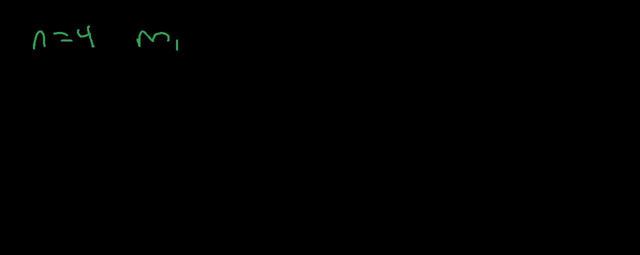 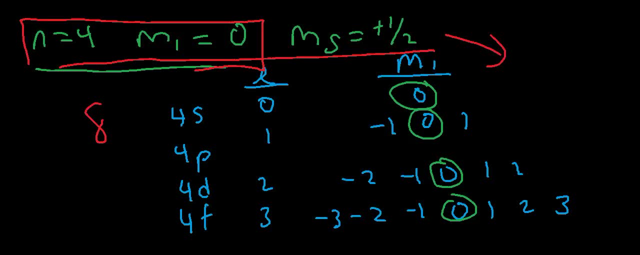 So in the 4th energy level we have a spin of minus a half. So in the 4th energy level we have a spin of minus a half quantum number. so the answer for this problem is there are four maximum and 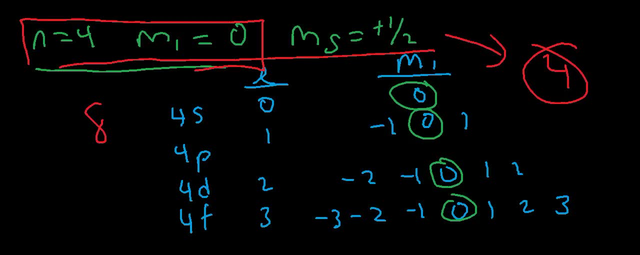 that electrons that can have an end value of 4 and mo value of 0 and a spin of plus 1 half. so hopefully you find this video to be helpful whenever you need to calculate the maximum number of electrons that has you know certain quantum numbers.